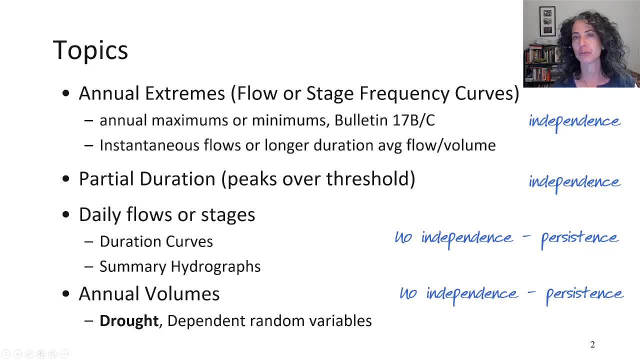 And if we choose that data set carefully, we can again assume independence. Then we move on to when we use all of the data. Daily flows cannot be considered independent of each other. They're persistent. Today's flow has quite a bit of dependence on yesterday's flow. 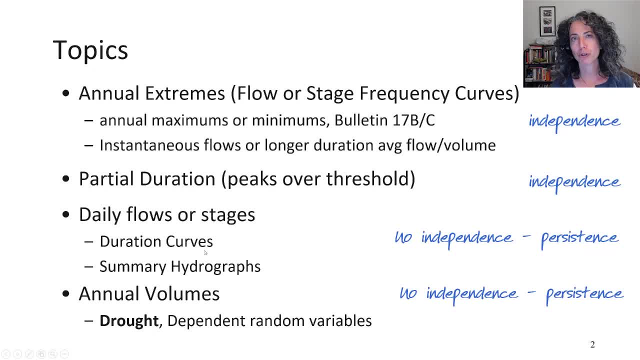 So we use different approaches. We're going to talk about duration curves and summary hydrographs And then finally, if we accumulate into annual volumes, again we have persistence And we're going to look at some modeling of dependent ramps. We're going to look at sampling of dependent random variables and use that as a chance to talk about drought. 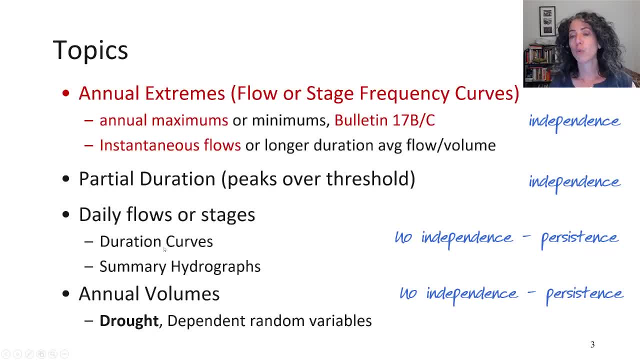 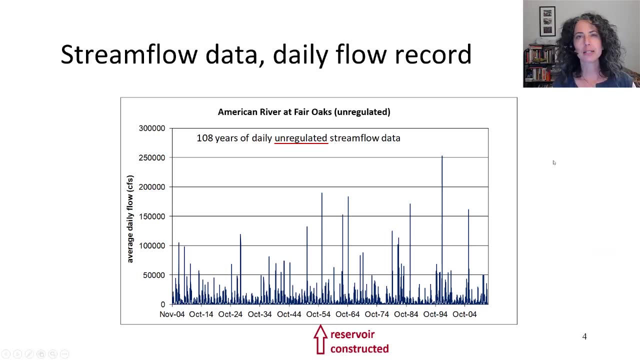 So in this first video we will talk about instantaneous annual maximums. We'll look at unregulated and then regulated flows, And with unregulated flows we'll take a moment to talk about Bulletin 17b. So this is a time series of flow on the American River in California. 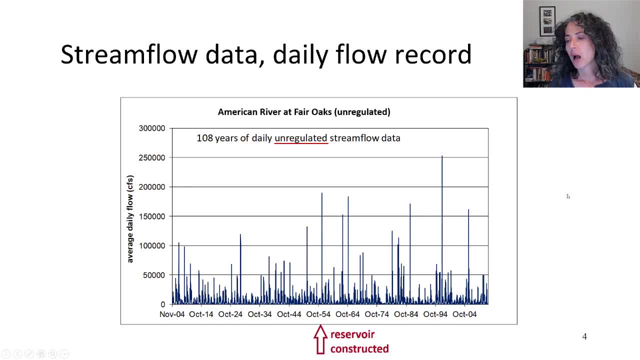 This is 108 years of record In order to have 108 years of unregulated flows. the first half of the record is just gauged flows And then a reservoir was constructed in the mid-50s, And so the second half of the record is back calculated unregulated flows based on inflow to the reservoir routed down to the gauge site. 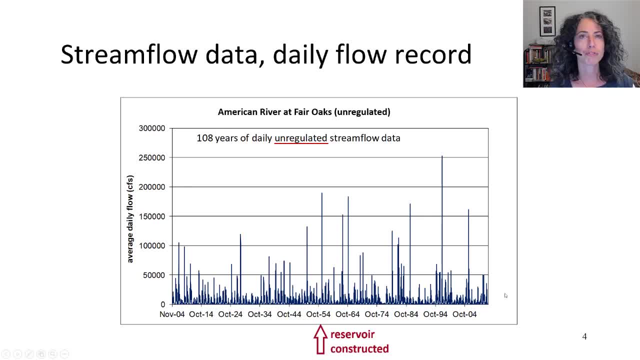 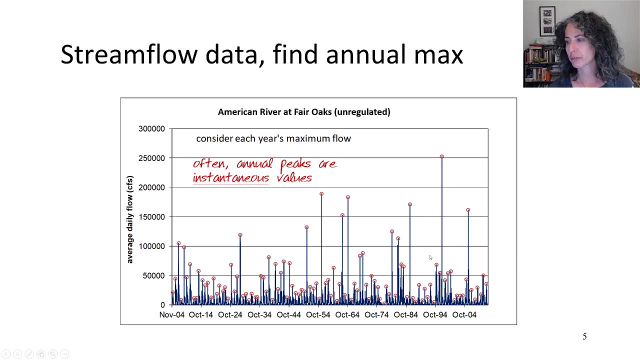 When I say unregulated flows, I just mean flow without human interference, And so we had to back out the influence of the reservoir. So to start with an annual maximum series, first we're just going to pull the largest value in each year. 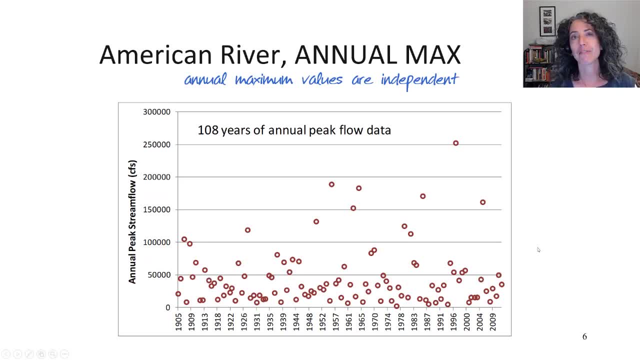 This is going to give us 108 values that we can use as a sample to estimate the probability distribution of the largest flow in each year, or the annual maximum. So let's take a moment to be reminded of the assumptions that we're making in this data set of 108 annual maximum series. 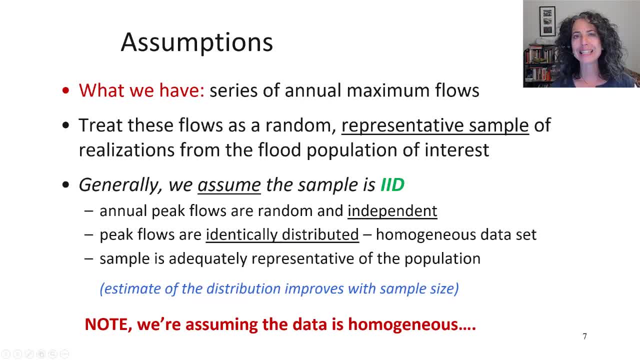 maximum values. So we're treating this sample as a random representative sample from the probability distribution of the largest flow in each year. We're assuming the sample is IID, which stands for independent and identically distributed. Identically distributed just means all the values either come from the same probability. 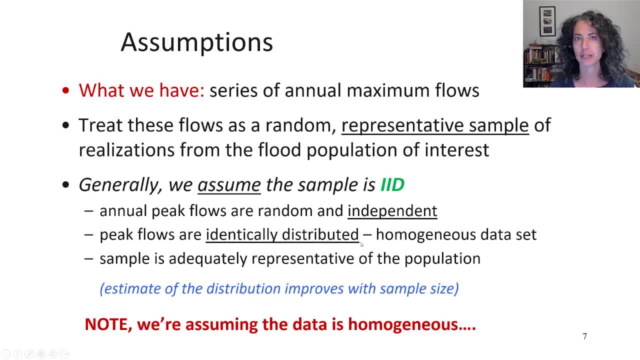 distribution or can be effectively represented by the same probability distribution. Another way to say that is: the data is homogeneous and because we collect data over time, the data is also stationary. We're assuming that the sample is adequately representative of the population, but at the 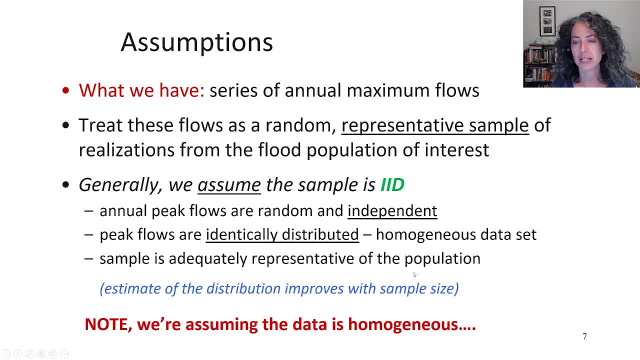 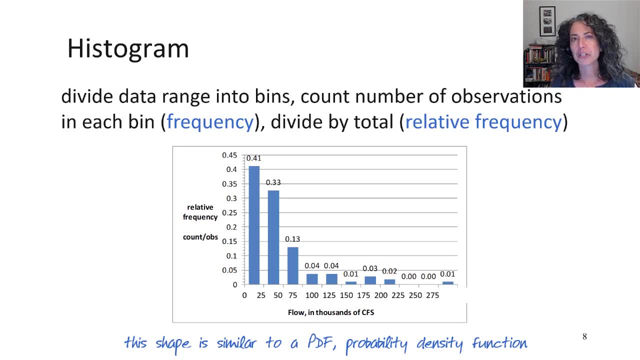 same time, we're keeping track of our uncertainty in that assumption and knowing that the estimate of our probability distribution is going to improve with sample size, And noting that the sample size we have is 108 years. So let's get a look at what this probability distribution might look like, based on our 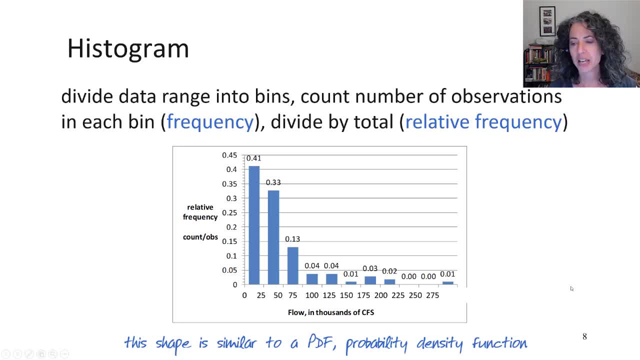 sample of observations. Here's a histogram of the data. We are seeing that most of our flows are here at the low end, and with a couple of values, though, that are many times greater than most of them. We saw in the introductory lecture that we can sometimes more effectively model flow. 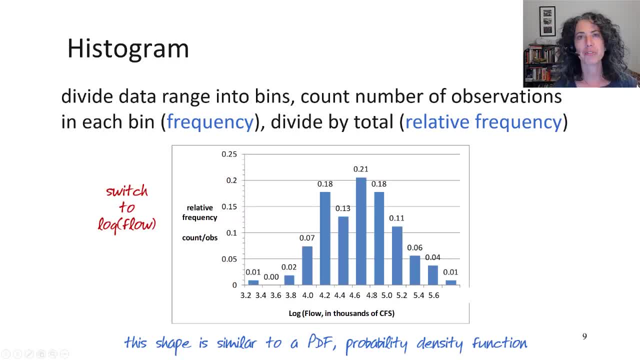 in log space. So here's a histogram of the base 10 log flows and, as we can see, it's a lot more symmetrical and friendly. So we're going to continue with flow in log space. So the histogram, as a reminder, is an estimate of the probability density function, or PDF. 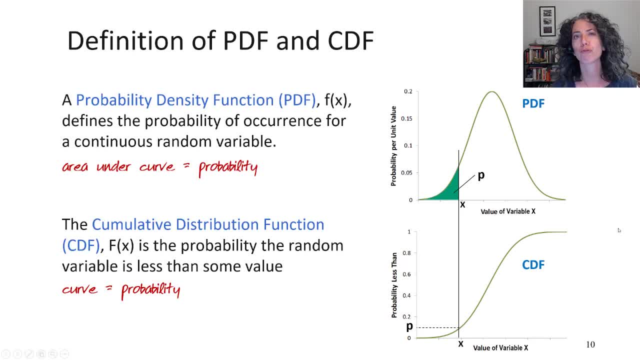 So a quick flashback to two of our forms of representing a probability distribution. We have the probability density function. here on the top, the bell curve form, where the curve shows us where the curve is high. We have the greatest probability density, meaning the greatest likelihood of seeing. 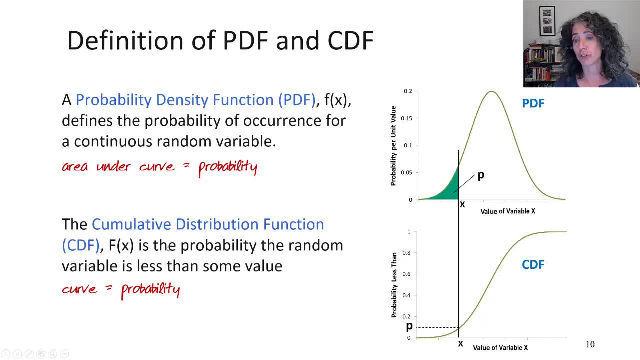 values of our variable in that range. The cumulative distribution function, or CDF, is just an accumulation of probability across the range of our variable ranges from 0 to 1.. It can be the probability less than. it can be the probability greater than. 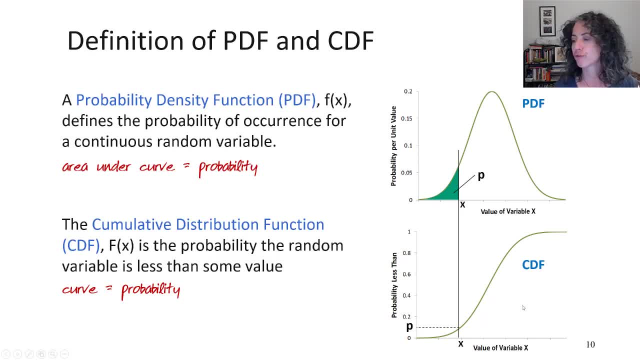 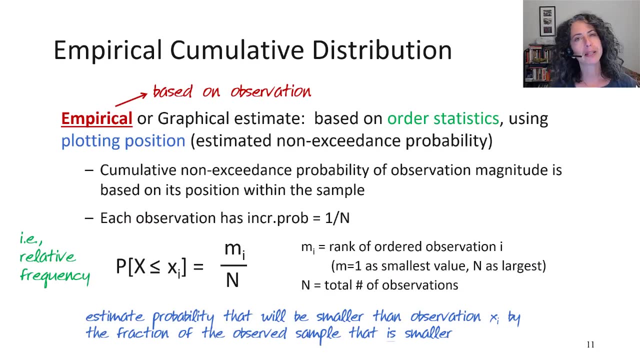 And we also sometimes show this in a frequency curve form with the axes reversed and adjusted, and we will walk through that. So if we want to estimate the cumulative distribution function with our data, we could choose to just accumulate the histogram, But instead. so we saw in the introductory lecture that it can be more effective to estimate. 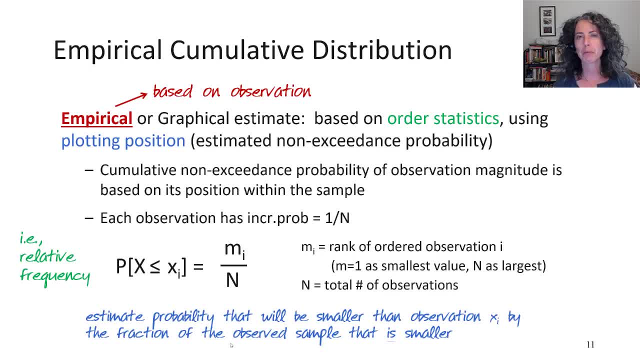 the cumulative distribution function by plotting all of the sample members versus plotting positions. So plotting position was just an estimate of the cumulative probability of each sample member and it's based on the sample size and on the position of each sample member or observation within the sample. that's been sorted by magnitude. 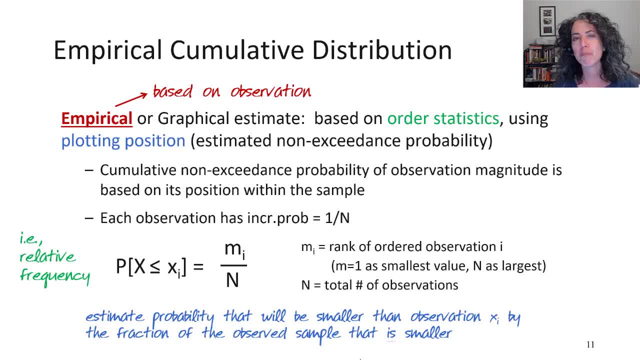 So effectively. we're just computing the relative frequency of being less than each sample member, based on how many of the observations were equal to or less than each observation. The rank is the count of observations that are less than or equal to, So m rank. 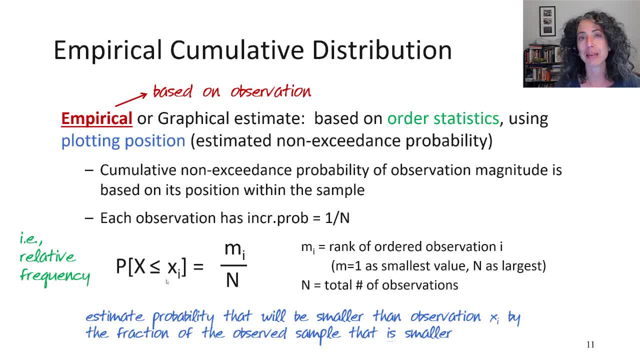 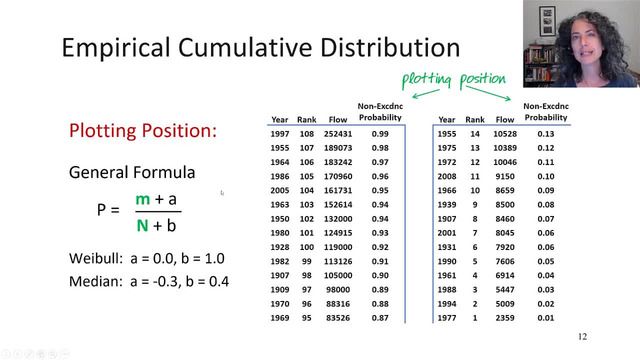 Over n. sample size is our estimate of the probability of being less than the sample member with that rank. So quick reminder: the plotting position is not quite as simple as rank over sample size, because either the largest or smallest value will have a rank of n and we'll get n over. 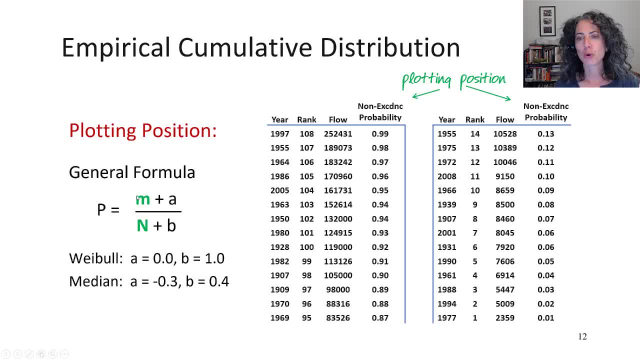 n equals 1, which is not a good probability estimate. So there are many plotting positions and each of them with an adjustment of rank over sample size. We look most often at Weibull and median. Each of the plotting positions- there's maybe a dozen others- aim at a certain characteristic. 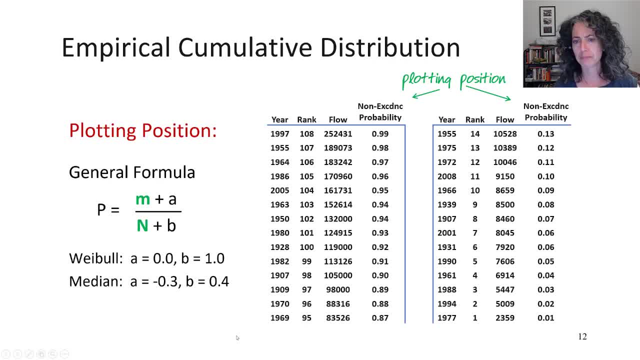 of the probability estimate. So for this example, we'll walk forward with the Weibull plotting position. What we have in the table is the largest 14 values and the smallest 14 values out of our 108, and they're sorted by flow. 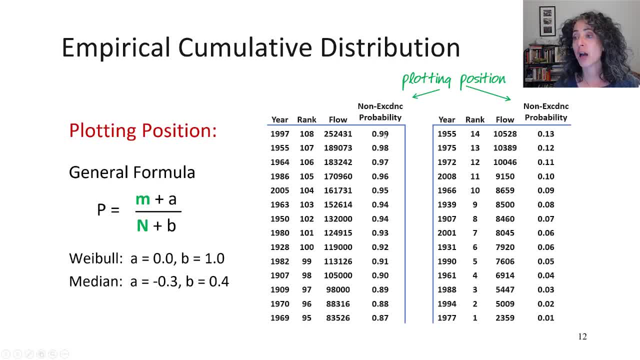 We see the rank, We see the computed plotting position, The non-exceedance probability. In this case, here's the smallest values with rank of 1 down here in computed plotting positions. So when I plot these I'm going to have a red circle around one of the points, just so. 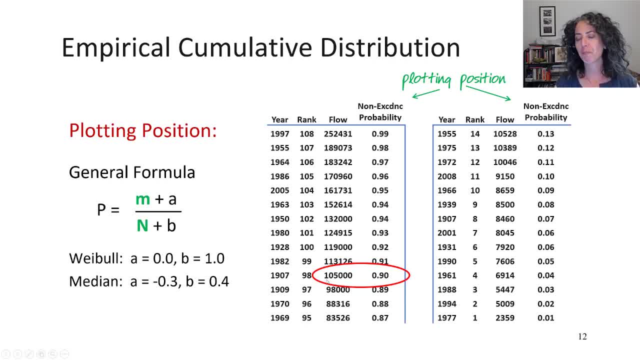 we can follow through the plots with their changing axes. So the value of 105,000 CFS has a non-exceedance probability estimate of 90%. We'll have that circled in each of the plots. So here's our data, plotted like the CDF shown here. 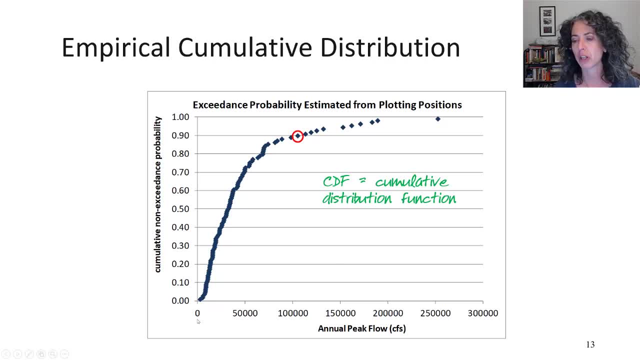 We can see that we have a 90% probability estimate. We'll have that circled in each of the plots. So we have the CDF shown in the previous slide, where we've got flow on the horizontal, we've got the cumulative probability on the vertical and here is our circled value at: 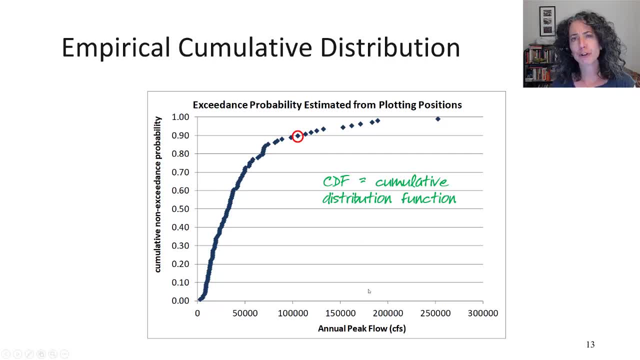 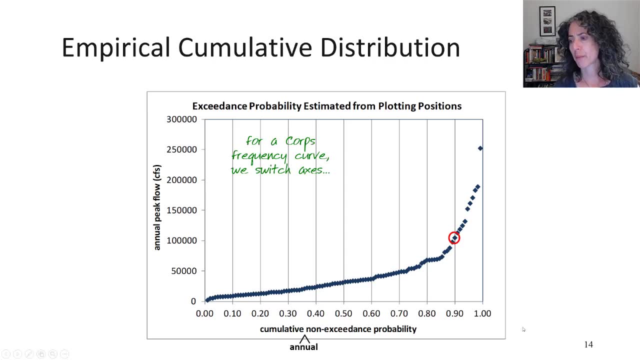 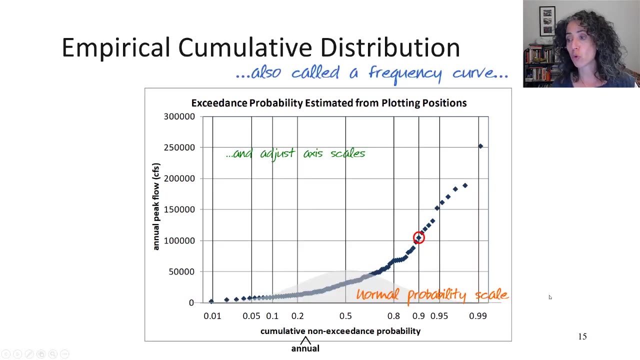 105,000 CFS To plot the frequency curve form. the first thing we do is we switch the axes. So we're going to put flow on the vertical and probability on the horizontal. We're going to switch this linear probability axis to a normal probability axis based on: 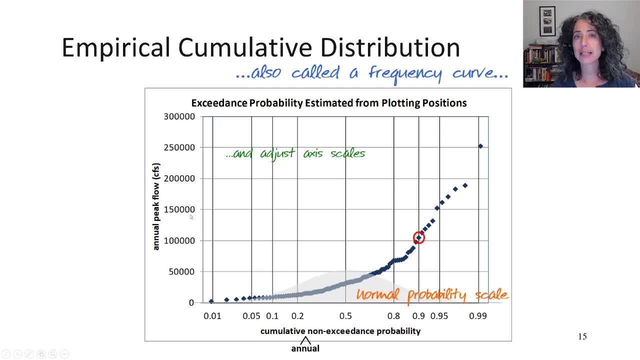 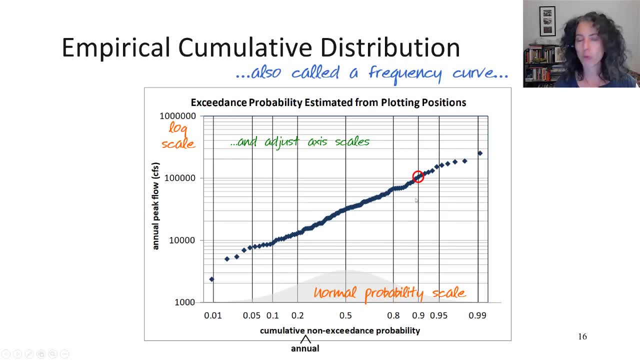 the normal distribution. We're going to change the flow axis from linear to a base-10 log scale, and now we see our data. We've still got this circled point over here. We see that our data is approximately a straight line. 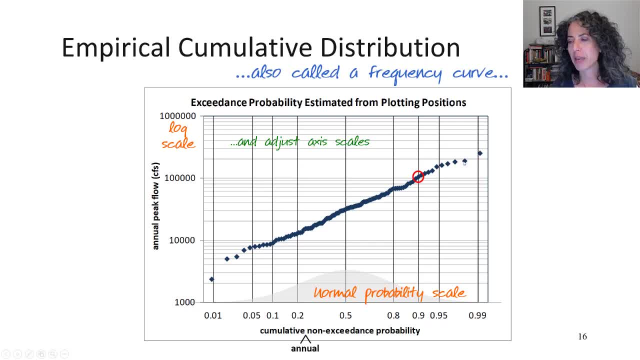 And that's not that surprising if we think about the histogram that we made of log flow. So a normal probability axis will show data as a straight line if that data is normally distributed, And so this is showing us that the base-10 log of our data is approximately a straight. 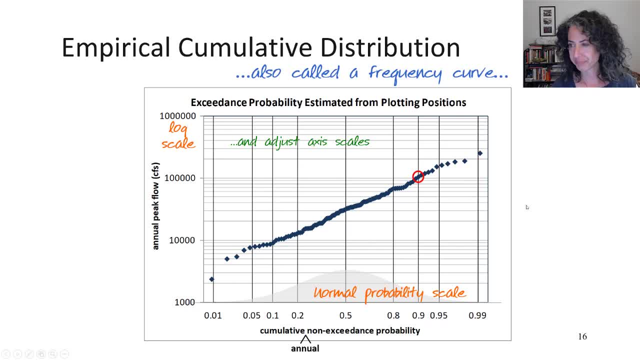 line. So how do we migrate written data in this region? Here's the data again. So I'll show you a graph that hết a log length every 3,000, 1,500 letters, and then the Army of is somewhat normally distributed. The next change we're going to make is to 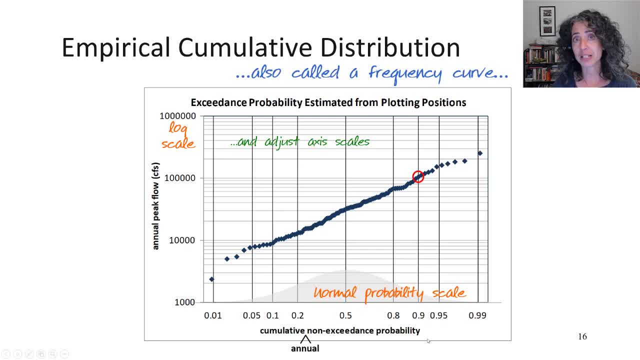 switch from cumulative annual non-exceedance probability to cumulative exceedance probability Right now. note: this is annual exceedance probability because we've got the largest flow in each year, right, so we're building annual probabilities based on that time step. Having gone to exceedance probability, we 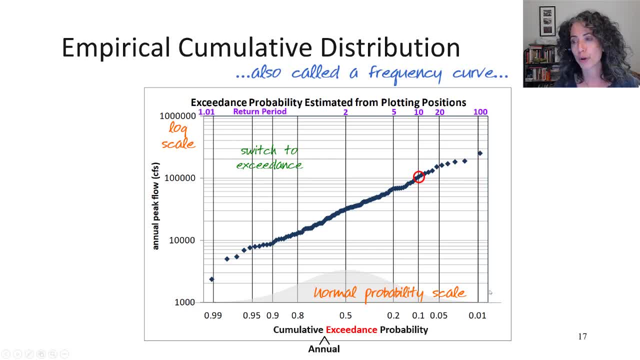 can plot return periods as well. The return period is just 1 over exceedance probability. So our value circled here. the 105,000 CFS with a 10% non-exceedance probability is just based on estimating that plotting position from the fact. 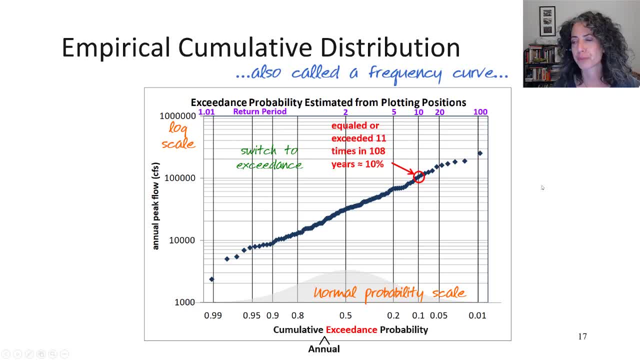 that the value has been equaled or exceeded 11 times in 108 years. right, and a similar assumption for our largest point is: we can plot it only by estimating that it was the largest value in 108 years. So what can we do next? 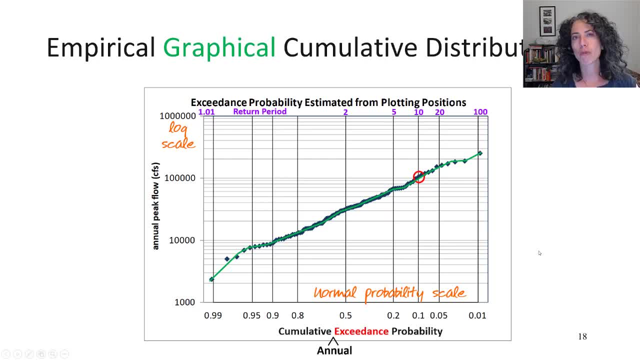 So what can we do next? Well, we can just draw a graphical probability distribution, which means I've just taken my pen to paper or taken my cursor to screen and drawn in a probability distribution. It does not have an equation, it does not have. 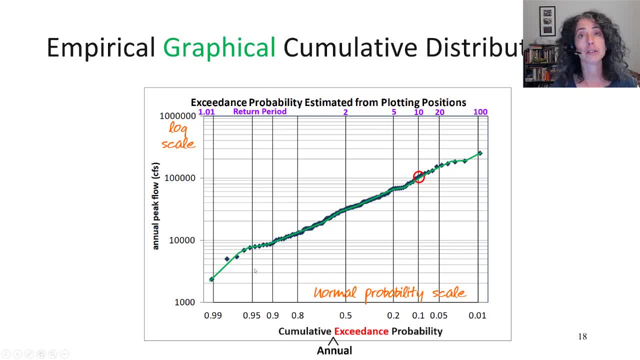 parameters. right, this is just a line And this can give us a good fit to our data, but the problem with it is, if we're interested in flow, we're not going to be interested in flows that are beyond the range of our sample. So another option: 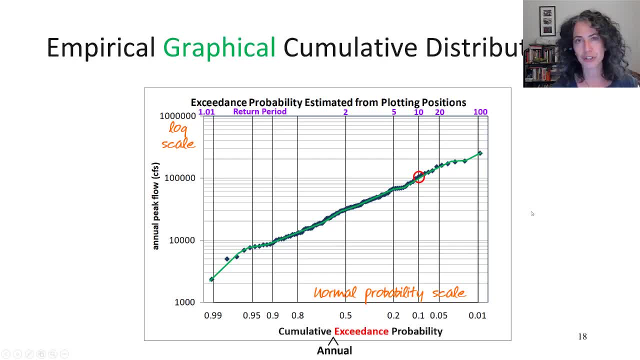 especially for unregulated flows that look this smooth is to fit an analytical probability distribution. So we can fit an analytical probability distribution, or what's called a parametric model, as you saw in the previous lecture, and this will allow us to take a quick look at our federal guidance for annual maximum unregulated 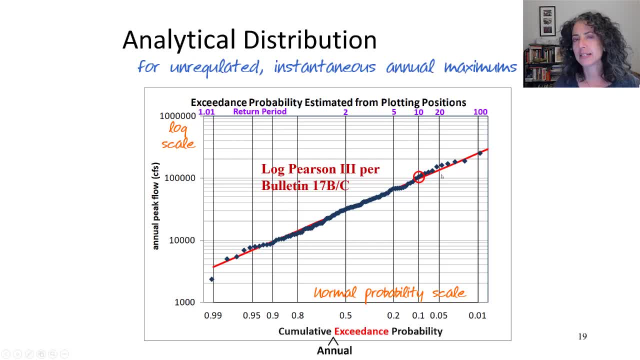 flows. So here this red line I've added is the fit of a log-Pearson type III distribution to our 108 years of annual maximum flow. I'm going to talk briefly about bulletin 17b and c, which is our federal guidance that suggests that we use the log-Pearson type III distribution. 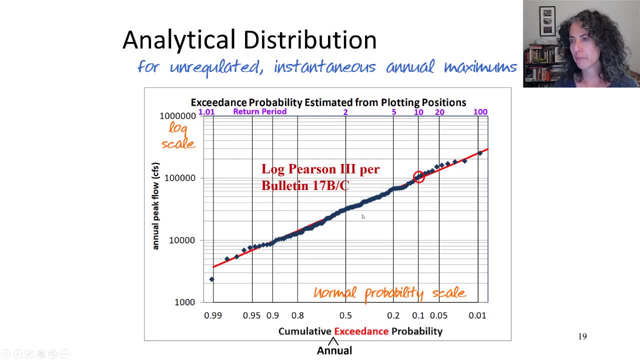 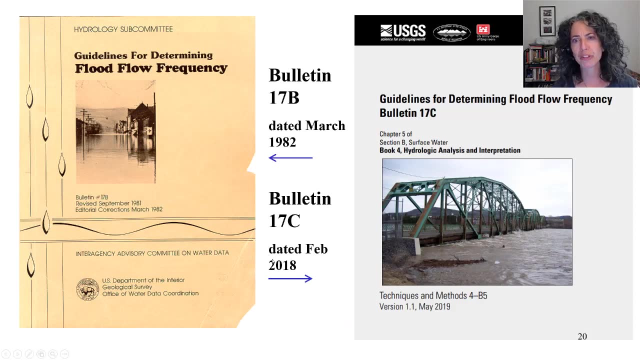 We're going to have a lecture later tomorrow, which is much more information about bulletin 17b and c. I will just say a few things about it here, because you're going to see it in workshop 9.. Number two, right. so bulletin 17b is the third or fourth in a series that was published. 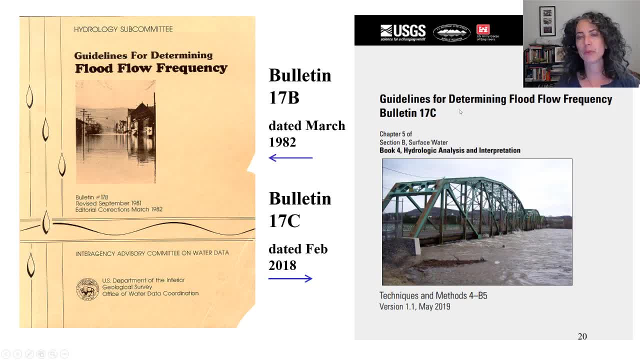 in 1982, and more recently now we have bulletin 17c, which we published in February of 2018.. The main difference between the guidance in 17c from b is the fitting method. We're still fitting the log-Pearson type III distribution, but we're doing it in a different way, Just. 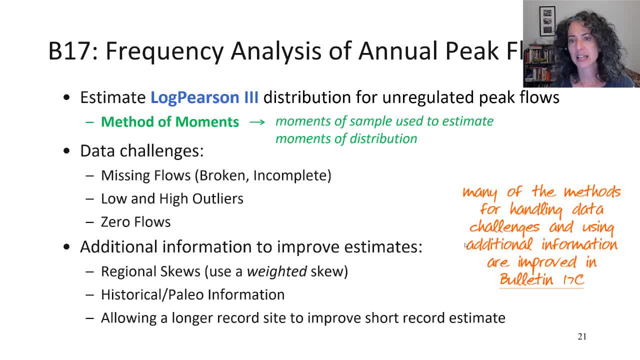 a few notes about the details about the bulletin 17 guidance. The federal guidance suggests that we estimate a log-Pearson type III distribution from the annual maximum series. suggests we use the method of moments to estimate that distribution, which, as a reminder, means we 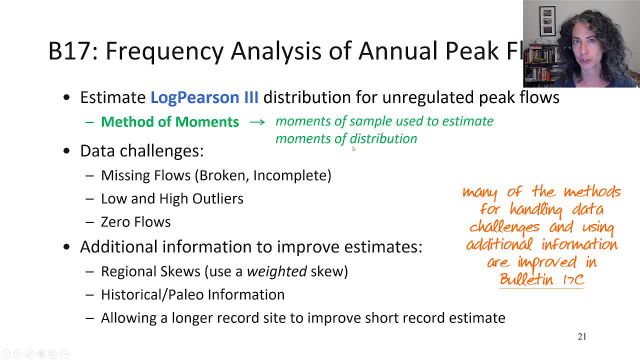 use the moments of the sample of data to estimate the moments of the distribution. Bulletin 17b does that with product moments. Bulletin 17c still uses product moments, but it uses an algorithm called the expected moments algorithm to do it. now there's more to the guidance than 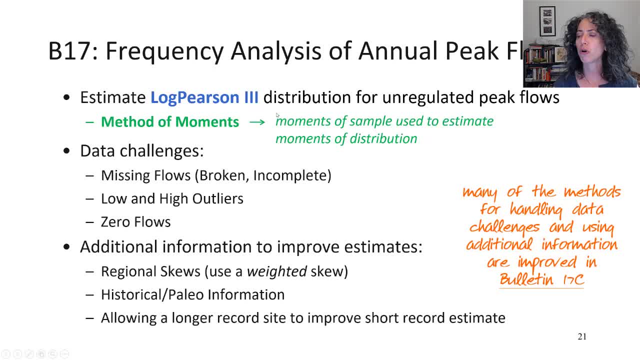 just saying which distribution to use on which data. there's also some adjustments to be made for difficult data, for example missing data or low or high outliers within the data set, and also for zero flows. zero flows are a problem because the logarithm of zero is undefined. but 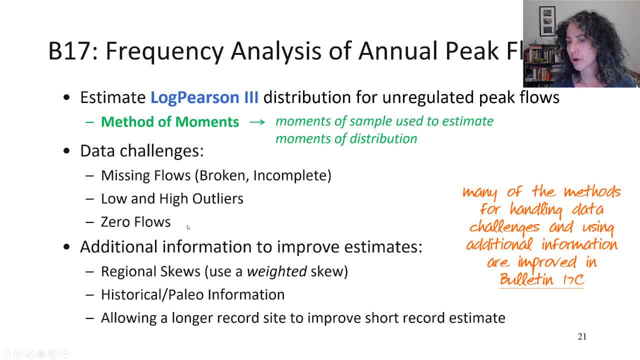 there are some streams that are dry for a few years in a row, and so the annual maximums are zero. so there needs to be a way to handle those, and that is part of the guidance. the guidance also allows us to use some additional information that can help improve the probability estimates. 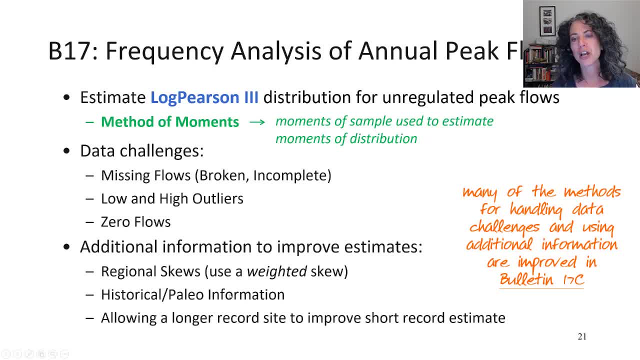 so if there's methods for using regional skews, for using historical or paleo information about large floods that have happened in the past or the fact that no large floods have happened in the past and there's also approaches for using longer record site nearby to improve the probability, 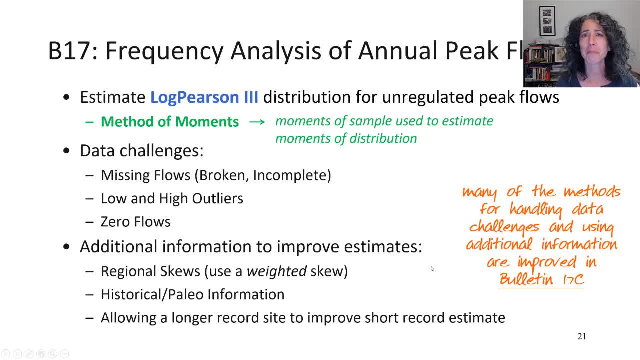 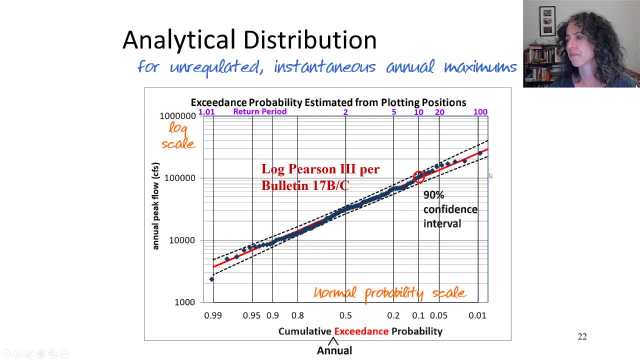 estimates for a short record site. all right, so that's all i'll say about bulletin 17 b and c for now, and we'll have another lecture on that later. however, one more thing that we want to include with our parametric model or our analytical probability distribution is some description of the uncertainty right, the 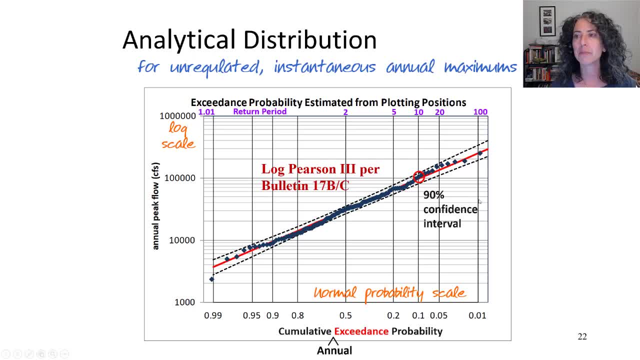 uncertainty here is based on the fact that we have a limited record that might not be representative of our distribution, and so we can draw, in this case, a confidence interval. simply put means we're drawing an interval that we believe has a 90 chance of containing the true. 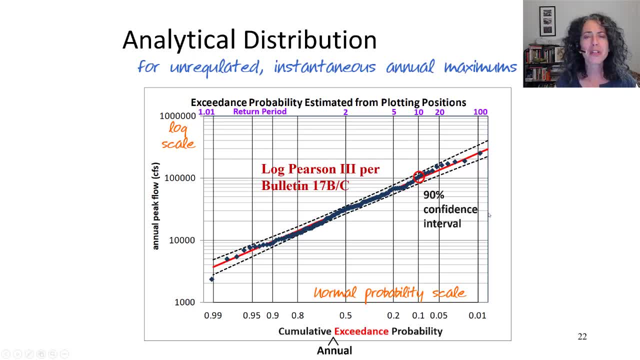 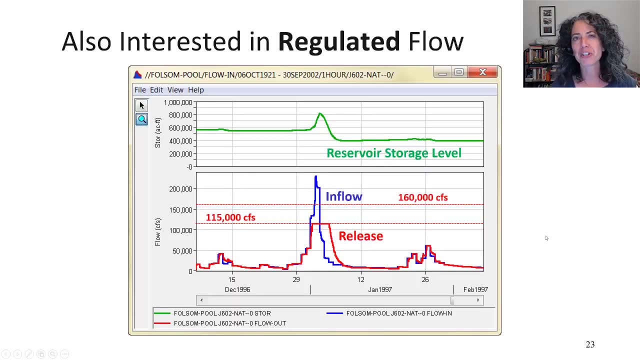 distribution right, so that's unregulated flows. i mentioned this site is below a reservoir, so we're also interested in the regulated frequency curve or the probability distribution of regulated flows right. this is a reservoir that holds a flood pool empty, so that when a large in-floor flood pool is, 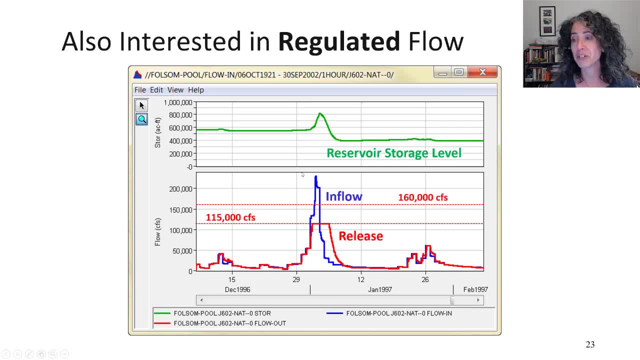 comes, the large inflows can be stored, increasing the level in the reservoir and holding the release- here in red- at a safe channel capacity until the inflow has dropped below that safe release, and then the water is continued to be evacuated at that release until the flood pool has been emptied. So we're 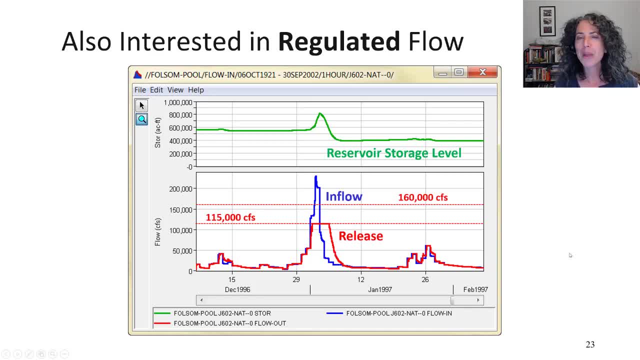 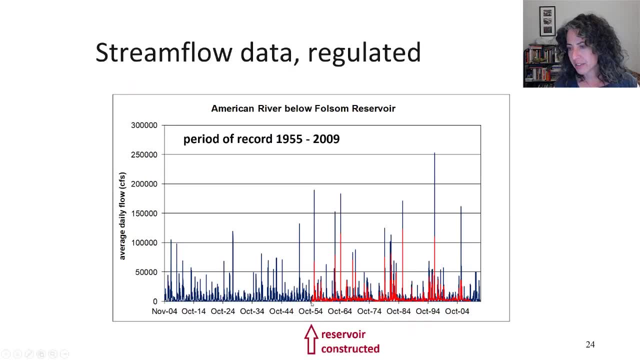 interested in building a regulated frequency curve, We can do it in the same way we did an unregulated frequency curve. We have a gauge record and the values in red are the gauged flows below the reservoir. so this is a shorter record from 1955 to well, in this case only to about 2005,- and we can pull out. 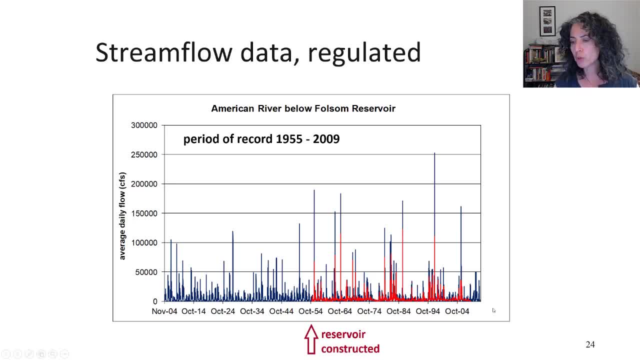 our annual maximums and do a frequency curve of this data. But we have two issues. the first is: are we looking at homogeneous data for the regulation, meaning, was the reservoir overcast or Was it pulled lava? Yes, and the biggest consolation for us is that if we look at these, counter ganhar wars. 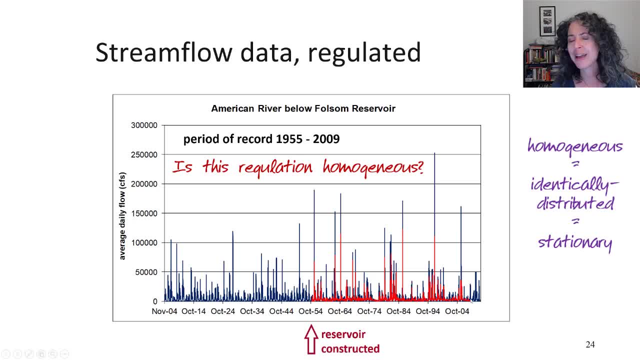 The ratio is going to matter for these two results. But we have two issues. The first is: are we looking at homogeneous data for the regulation meaning? was the reservoir always Då they still buildish? the reservoir operated in the same way for this entire period and it's fairly common. 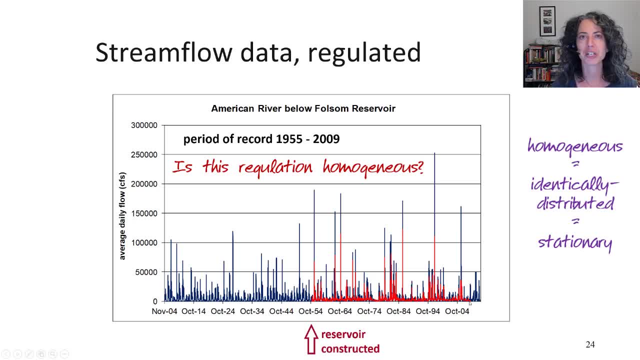 that it would not be So. if the operation isn't homogeneous, then we don't have a homogeneous sample, meaning it's not identically distributed, it's not stationary. Another issue is that this is a shorter record. This is a 50-year record as opposed to the 108-year record. 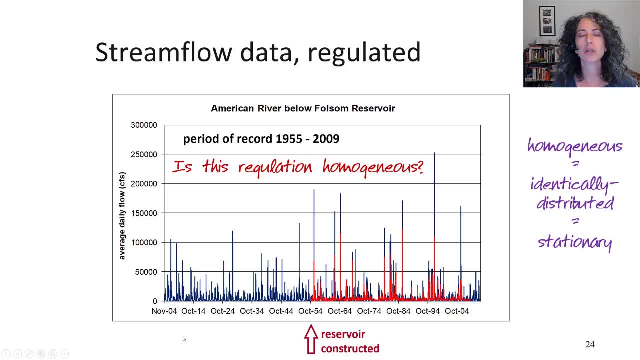 So one way we can handle both of these issues is to use a reservoir simulation model which can simulate current reservoir operations, and then we can route our entire period of record of data through the reservoir simulation model. That will allow us to be sure we have current and homogeneous regulation, and it will also 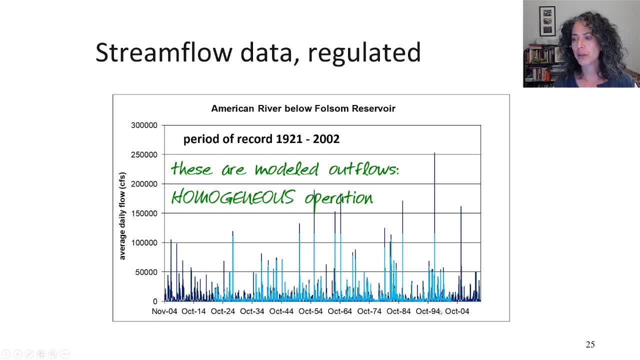 give us a larger data set. So here in light blue, we have simulated reservoir releases routed to the downstream location from the reservoir simulation model. Now it isn't actually the entire data set, It's the entire period of record that got simulated. 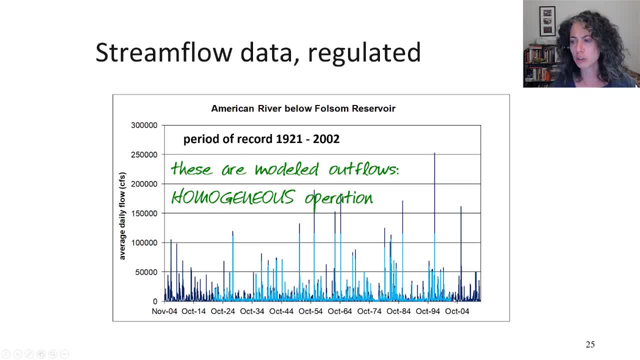 It's only 81 years of the period of record, But it is still longer than the original gauged flows and it is a consistent operation. So, in the same process as with the unregulated flows, we're going to pick out our annual 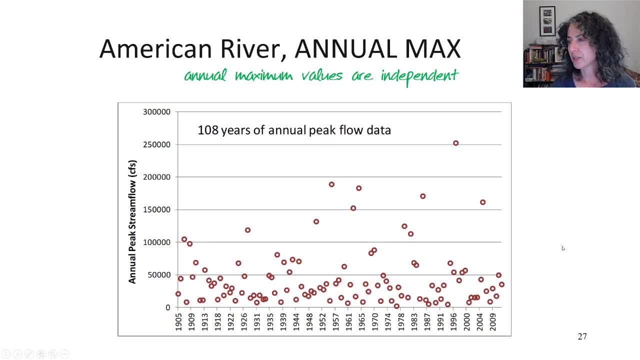 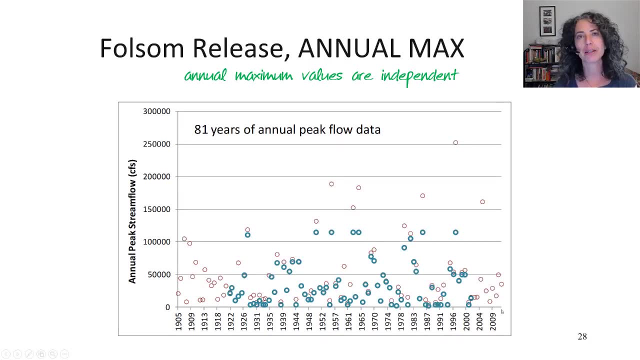 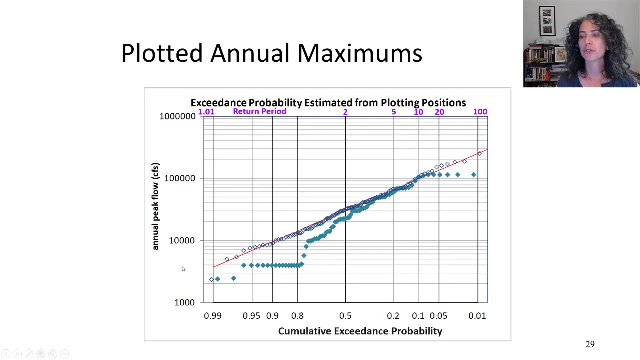 maximums. Our data set now, instead of being these 108 annual maximum unregulated flows, we're going to have 81 regulated maximums And we do a frequency analysis of those by sorting them, ranking them and plotting them against plotting positions. 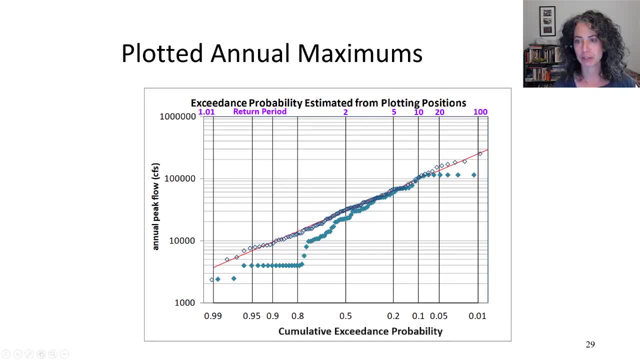 So our original unregulated flows are now the hollow diamonds and the blue is our regulated flows. Now we can see a little bit more clearly now that we've got some thresholds. This lower threshold at 4,000 CFS is, I think, hydropower flow. 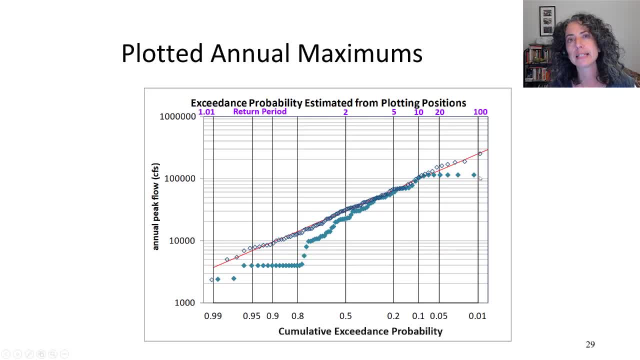 This upper threshold at 115,000 CFS is that channel capacity, And what we're seeing here is that we've got some thresholds, And what we're seeing here is that we've got some thresholds, And what we're seeing here is that in our period of record there weren't any events. 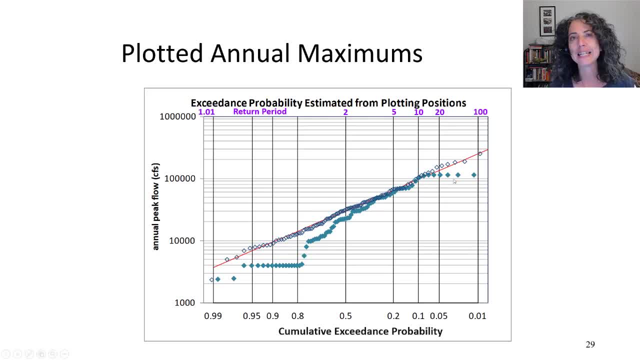 large enough for the volume to have exceeded the flood pool in the reservoir and called for a release beyond the channel capacity. So we only have flows that are topped off at this 115,000 CFS. So what should we do next here? Well, with the unregulated flows we fit an analytical probability distribution. 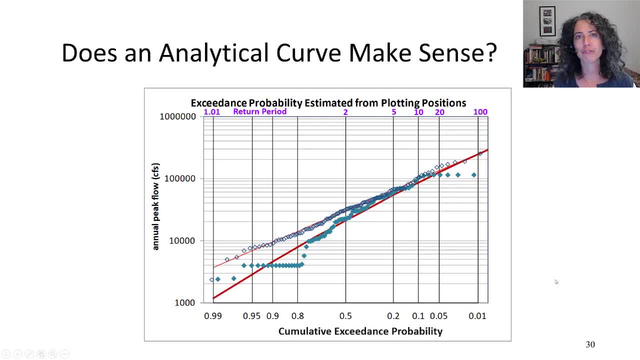 What would happen if we did this to these. Here's an analytical fit of a log Pearson type 3 distribution And what would happen if we did this to these. Here's an analytical fit of a log Pearson type 3 distribution And what would happen if we did this to these. 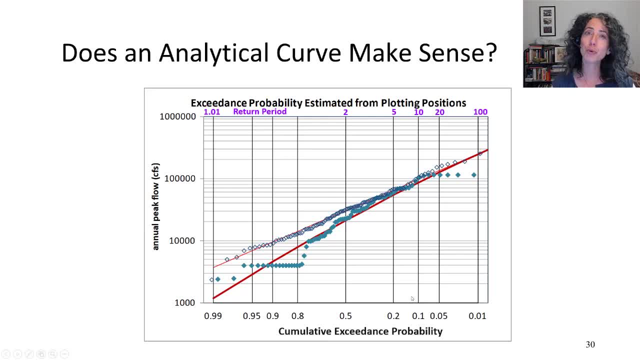 Here's an analytical fit of a log Pearson type 3 distribution. We can see that this distribution does a very nice job of smoothing through our data but therefore does a fairly poor job of respecting the thresholds. down here at 4,000, up here. 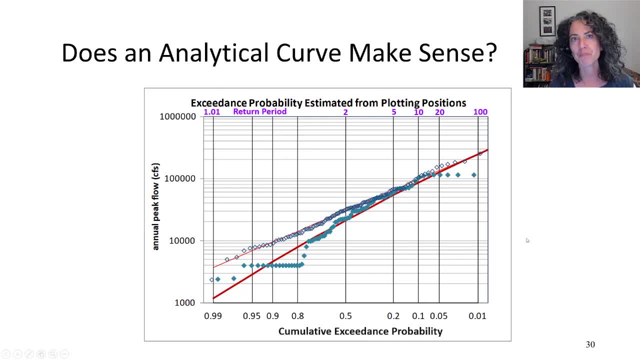 at 115,000.. So this is not at all a good representation. In the case of regulated flows it is a better idea to use a graphical frequency curve So I can draw it flat at relevant thresholds. I can smooth through some data points. 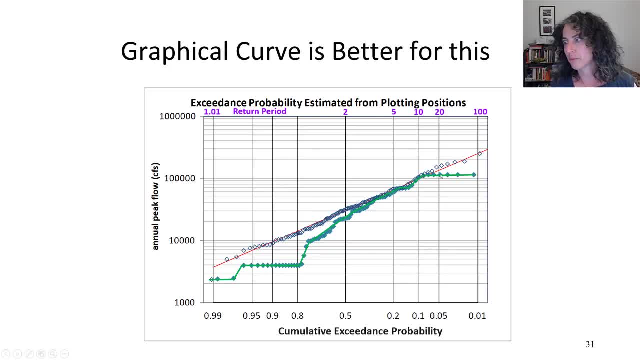 If I think there's sampling error. but I can go flat again and respect a threshold up here, right? So a graphical curve is a better approach, but it does leave us the problem of what to do beyond the range of the data, right. 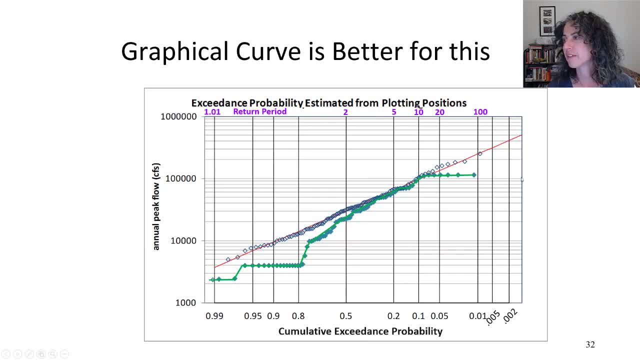 If we're interested in larger events with lower probabilities. we don't really have a method to extrapolate here. right, We have a range that we need to make estimates on the probability distribution. What we generally do here- Okay, So what we do here is we go back to our reservoir model with some synthetic hydrographs. that 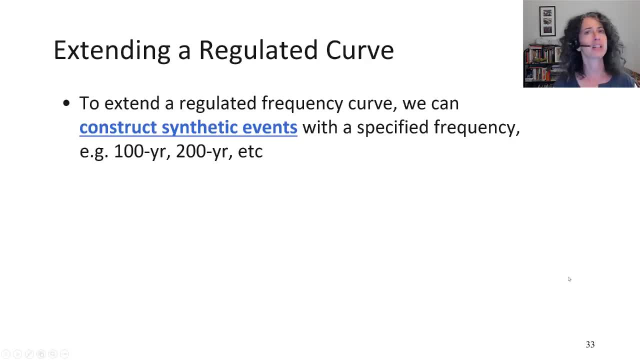 are constructed to have a particular exceedance probability, right? So this is going to be the topic of our next video, right? So we're going to construct synthetic events that have a specified frequency. The way we do this is to estimate families of frequency curves that are longer duration.